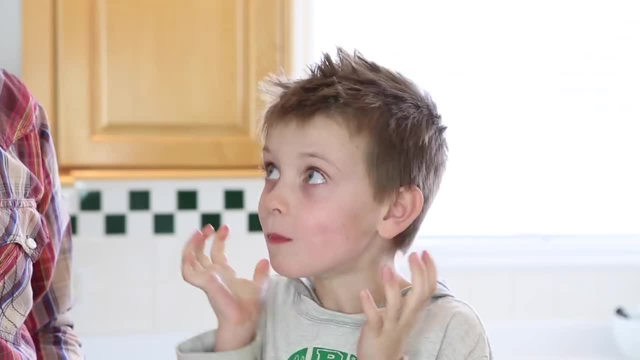 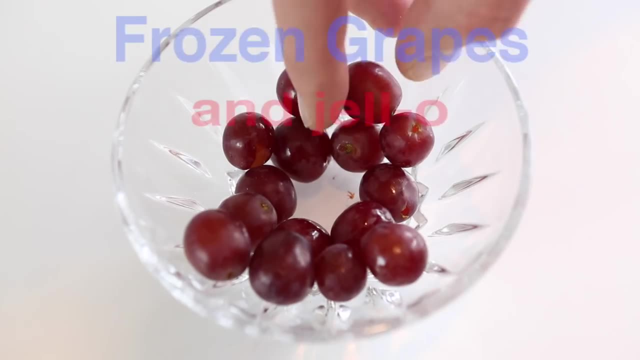 Alright, Lucky Lucas is our second taste tester. Watch out for the brain freeze, Lucas. Oh, you got it. Sorry, buddy. Well worth it, though. That's my second thumbs up. Alright, this last one's a simple one, but it's really good. 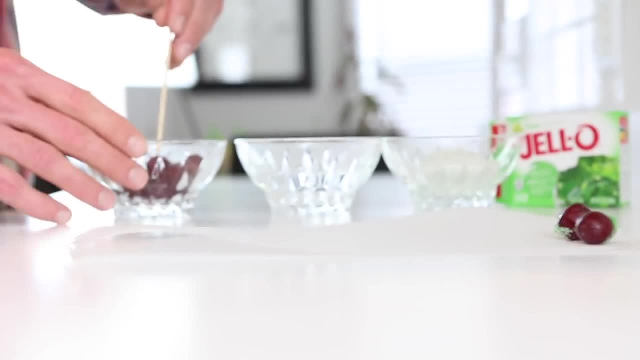 Take some grapes, Dip them in a little water, Dip them in a little juice, Put them in a little Jello mix, Put them on a plate, Freeze them. This one has to get thumbs up. Going three for three here. Try them out, kiddos. 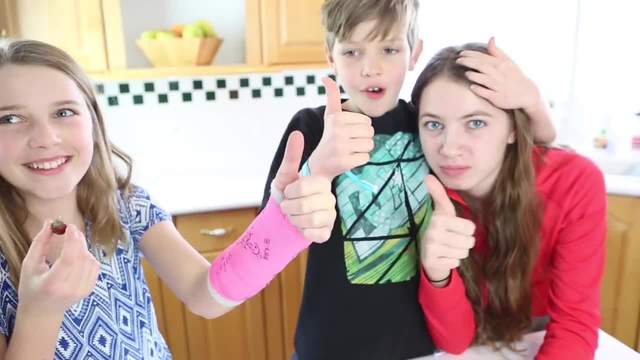 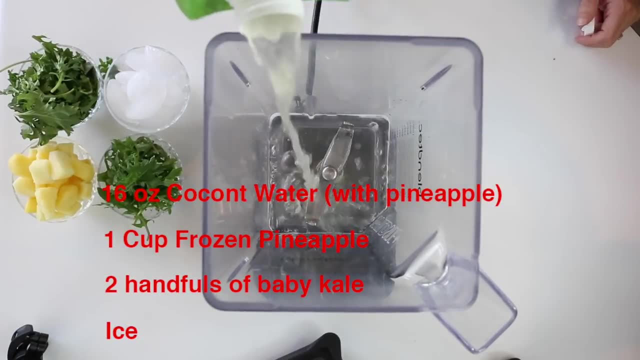 Let's see what they say. Hope they like them. Alright, thumbs up All around. My turn, My turn. First up: pine kel-lata- Kind of like a pina colada, but with kel instead. So you're going to use some coconut water with pineapple and you're going to put two 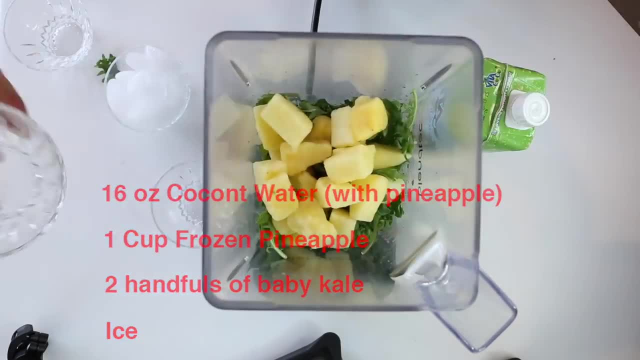 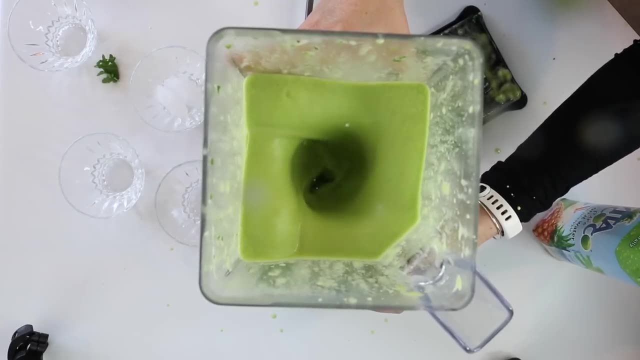 handfuls of kel in some frozen pineapple and some ice. Then go ahead and blend it up and it's going to be the consistency of a pretty thick smoothie. And look how thick it is. Wow, That pops out of the blender. 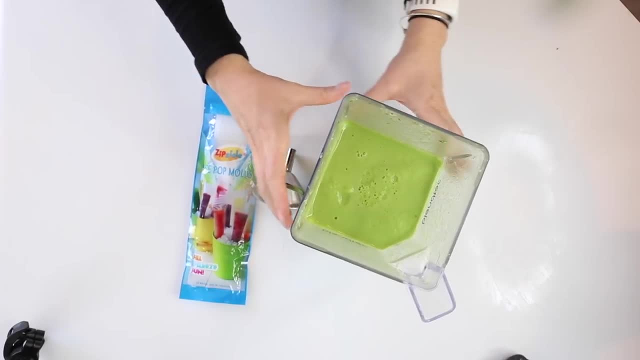 Make sure you keep the lid on. Now here's the fun part: Putting them in little baggies So the kids think they're little frozen popsicles. I found these little bags on Amazon and just put them in and freeze them. 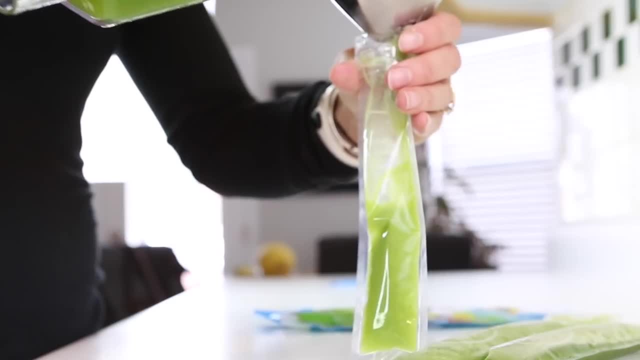 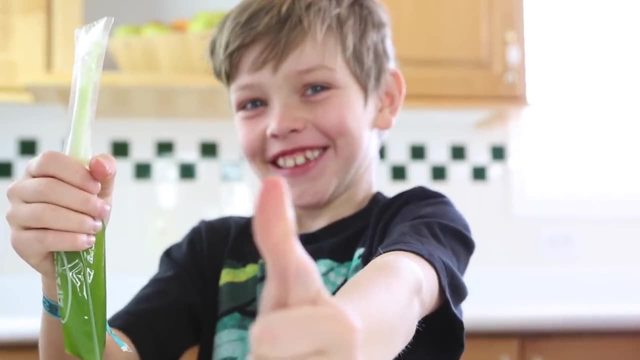 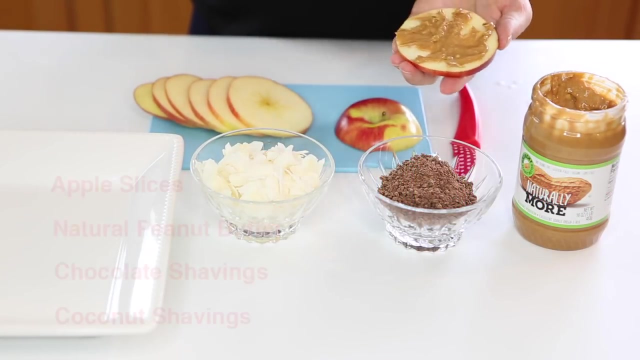 You can see the reaction on this one. My first thumbs up. Number two: apple cookies. Alright, heads up. This is so good You'll want to eat all these. Take some apples, Slice them in thin slices. I didn't take out the core because we kind of eat around the core, but you can pop out. 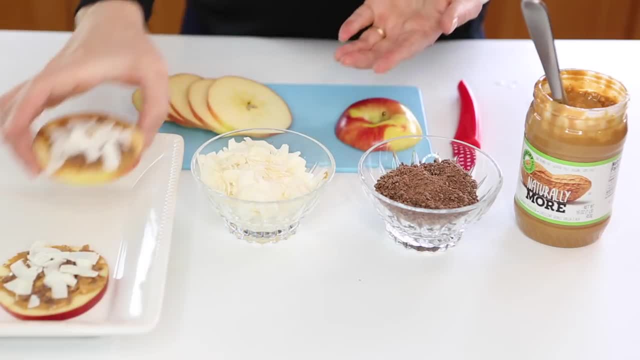 the core. It's so good, I'm going to add some natural peanut butter, some chocolate shavings and some coconut shavings, and all these are delicious, While the competition's hot. Jared's got three and I've got one. 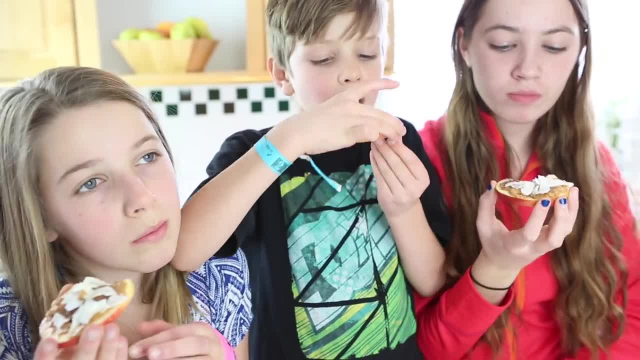 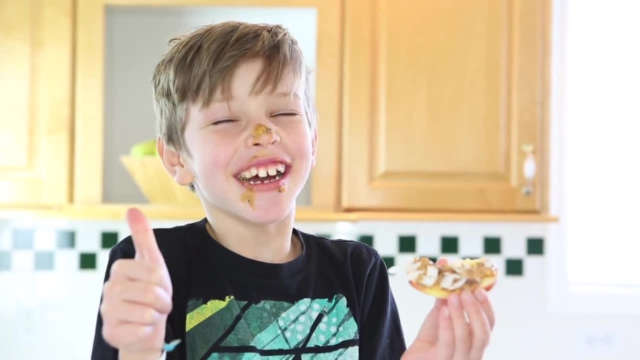 I'm hoping for my second thumbs up. Come on, guys. Yay, Second thumbs up. This one can get a little messy, but it's well worth it. The kids absolutely love these apple cookies. Last one: coconut water: fruit pops. 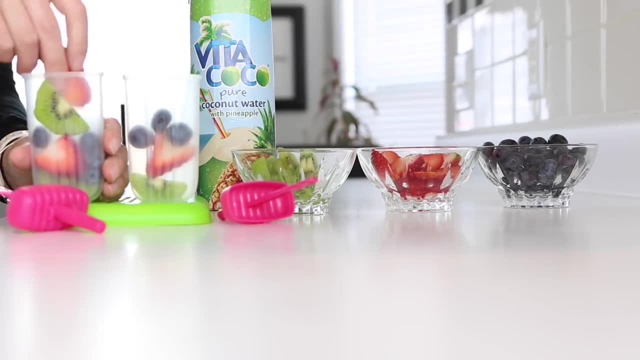 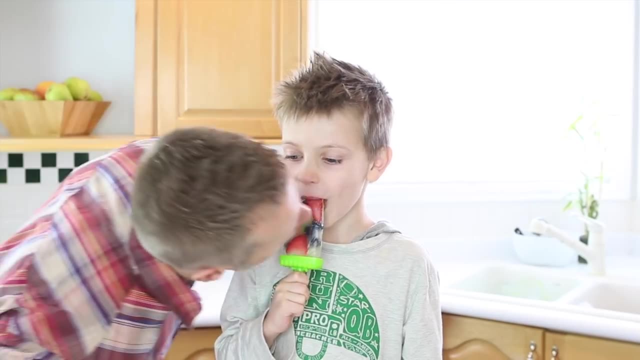 Get your popsicle molds, Fill them full of fruit. fresh fruit chopped very thick, Chop very thin, Fill up with coconut water and freeze. Luke, you're my tie breaker, or tire, What's it going to be Woo? 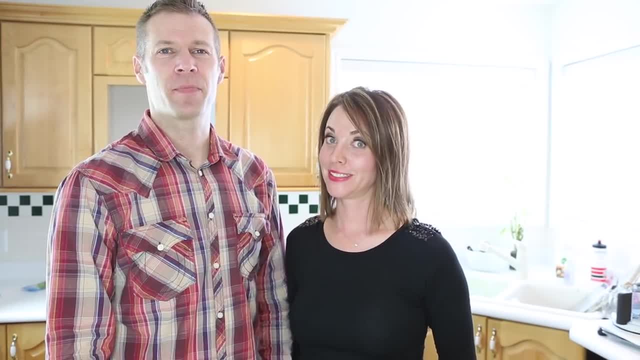 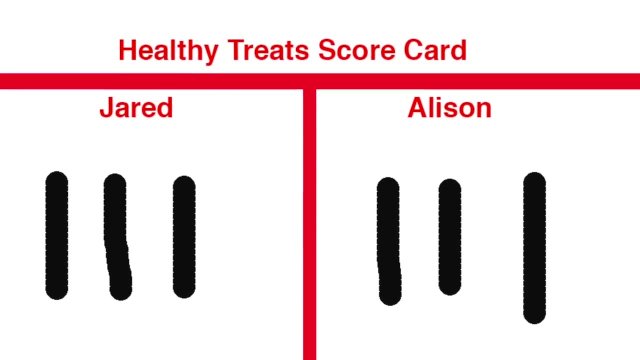 Thumbs up. Alright, so I think we've got our snack challenge all wrapped up. It seems like it went well. The kids are still eating in the background- Yeah, they are, And I think I won. I got three out of three thumbs up.